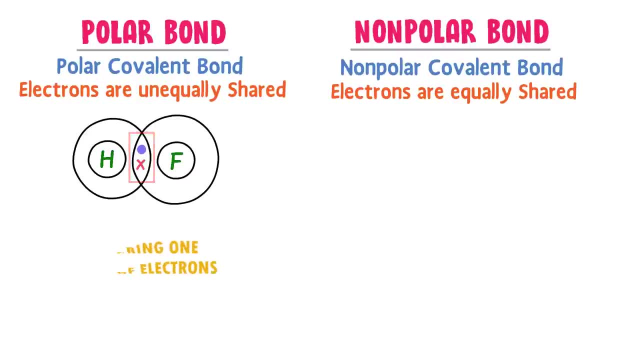 by sharing one pair of electrons. Now listen carefully. Fluorine atom is more electronegative than hydrogen. It means that fluorine atom pulls the shared pair of electrons more towards the opposite direction. So if hydrogen fluoride forms a covalent bond, 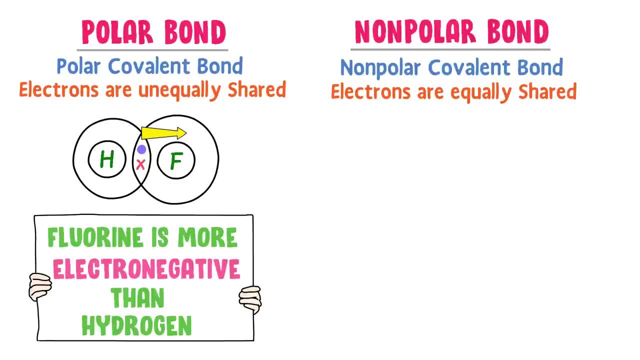 then hydrogen is more electronegative than hydrogen atom. Due to this electronic cloud tilt more towards fluorine atom than hydrogen. As a result, partially negative charge appears on fluorine atom and partially positive charge appears on hydrogen atom. Therefore we say that 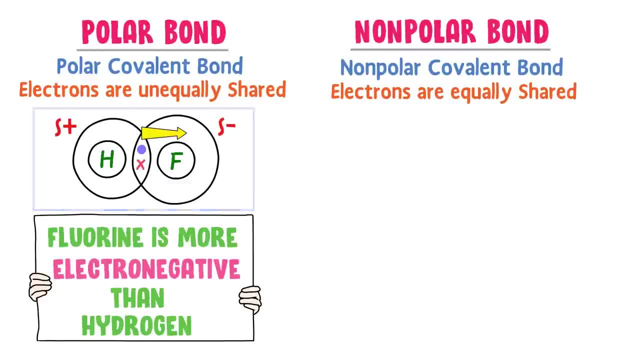 the bond between hydrogen and fluorine is polar, because this molecule has positive pole and negative pole. Now consider a chlorine molecule. Chlorine atom forms a covalent bond with other chlorine atom by sharing one pair of electrons. Both the chlorine atoms pull the shared pair of electrons equally on either side. It is because 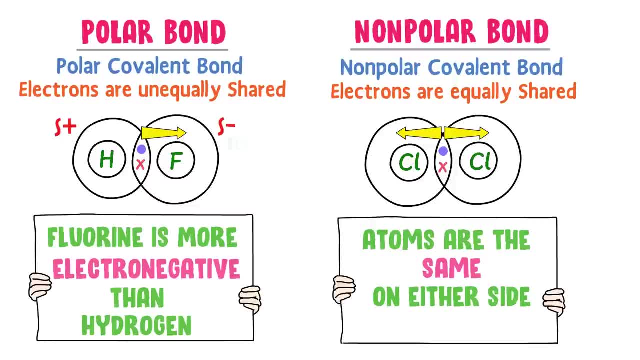 atoms are the same on either side, So the electronic cloud remains in between. As a result, no partial negative and positive charge appears on either side. Therefore, the bond between these two chlorine atoms is a non-polar, because this molecule doesn't have positive pole and negative pole. Now how can we tell if a molecule is polar? 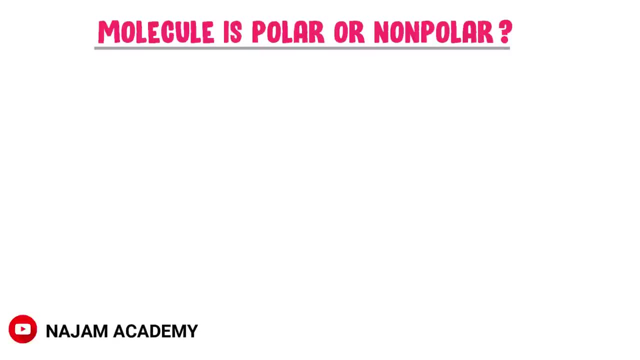 or non-polar. There are two factors that determine the polarity of a molecule. The first factor is electronegativity difference and the second factor is net dipole moment. If electronegativity difference is greater than 0.5, we call it a polar bond. If electronegativity difference 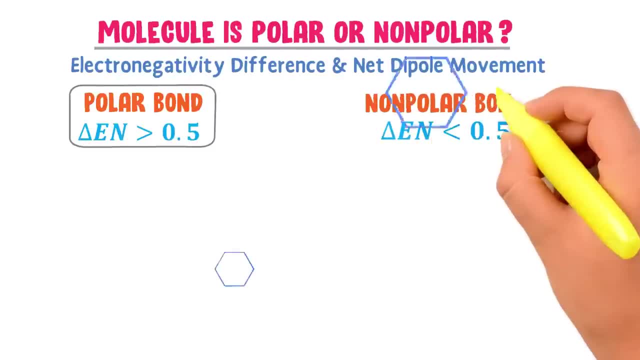 is smaller than 0.5, we call it a non-polar bond. For example, consider a molecule of HCl. The electronegativity of chlorine is 3.0 and the electronegativity of hydrogen is 2.1.. When we calculate the electronegativity difference between hydrogen and chlorine, 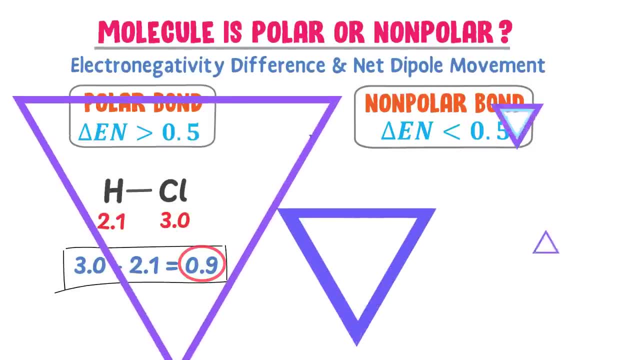 we get 0.9.. 0.9 is greater than 0.5.. So partial negative charge appears on chlorine and partial positive charge appears on hydrogen. Hence we say that it is a polar molecule due to positive pole and negative pole. Here consider a molecule of chlorine gas. The electronegativity 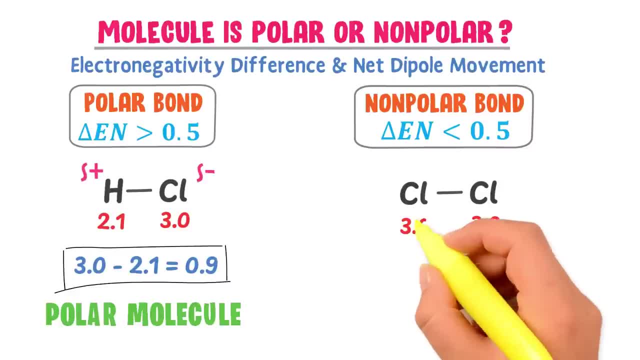 of a single chlorine atom is 3.0.. we find the electronegativity difference between these same chlorine atoms. we get zero. This electronegativity difference is smaller than 0.5. So it is a nonpolar bond. Therefore we say that: 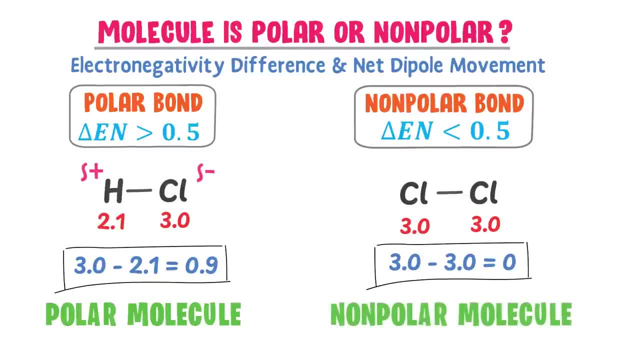 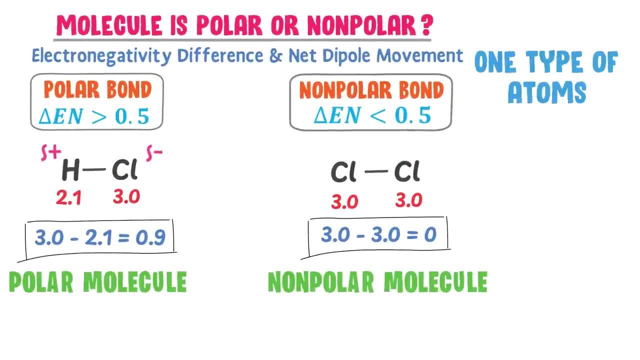 chlorine molecule is a nonpolar molecule. From this example we learn that if molecules are made up of one type of atoms, they are nonpolar molecules, Like molecules of nitrogen oxygen, fluorine, bromine, iodine, etc. Now let me give you some difficult examples of polar and nonpolar. 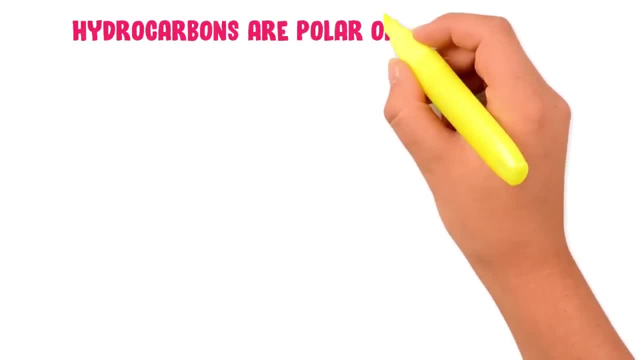 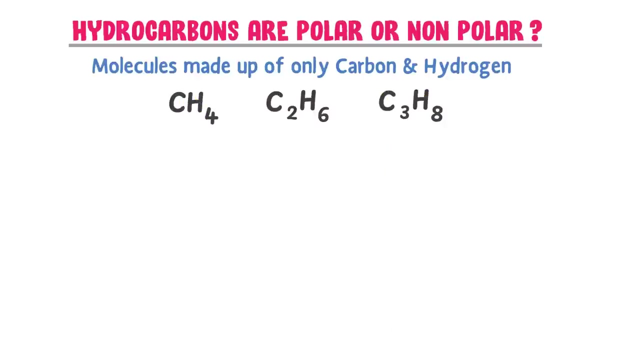 molecules Are hydrocarbons, are polar or nonpolar molecules? Well, hydrocarbons mean molecules only made up of carbon and hydrogen atoms, Like methane, ethane, propane, etc. Firstly, we check the polarity of carbon and hydrogen bond. The electronegativity of hydrogen is 2.1 and the electronegativity of carbon is 2.5. When we 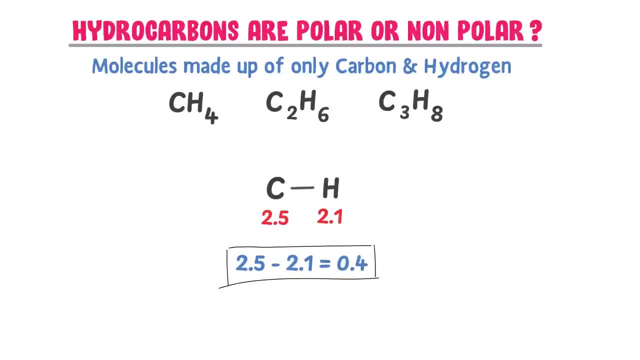 calculate the electronegativity difference between these two atoms, we get 0.4.. It is less than 0.5.. So the carbon and hydrogen bond are nonpolar. So we get 0.5.. So the carbon and hydrogen bond are. 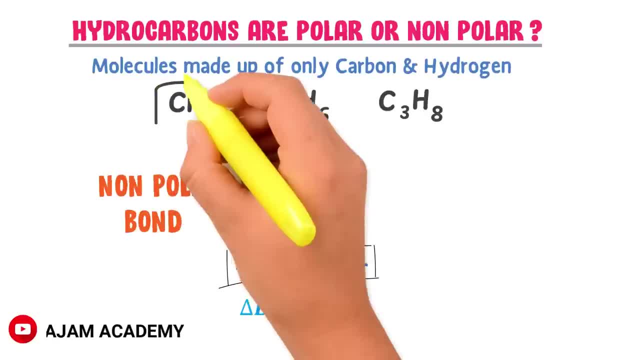 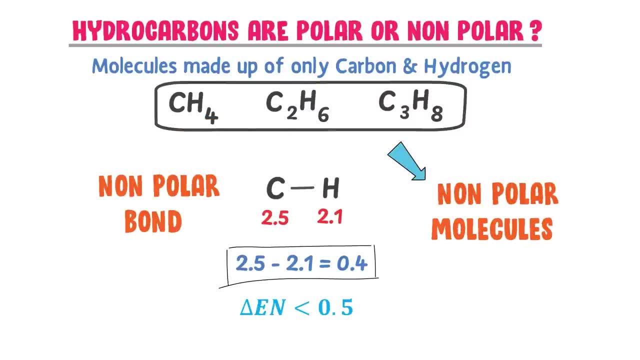 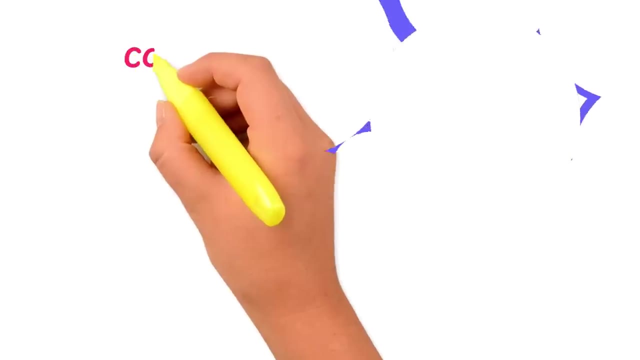 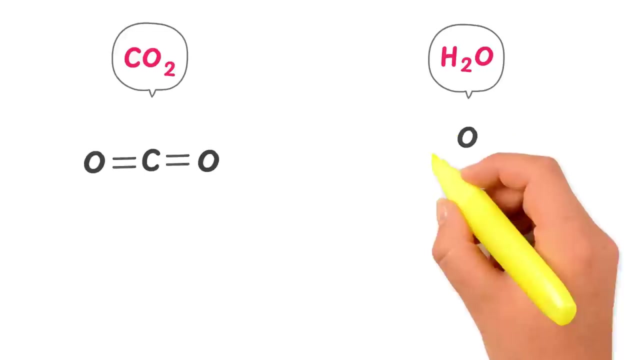 nonpolar. Therefore, we say that all hydrocarbons like methane, ethane and propane are nonpolar molecules, Because the bond between carbon and hydrogen is nonpolar. Now what about the polarity of carbon dioxide and water? The structure of carbon dioxide is linear and the structure of 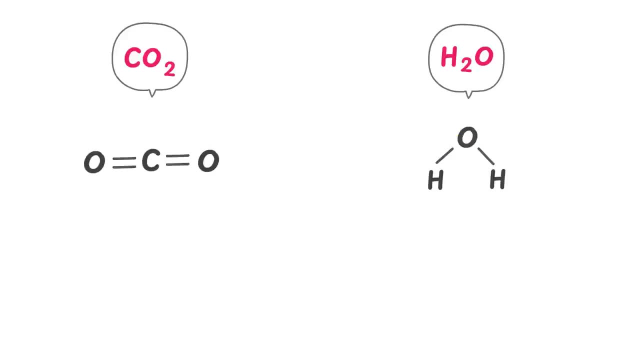 water is bent. Here the electronegativity of oxygen is 2.1 and the electronegativity of hydrogen is 3.5.. And the electronegativity of carbon is 2.5.. The electronegativity difference between them is 1.. 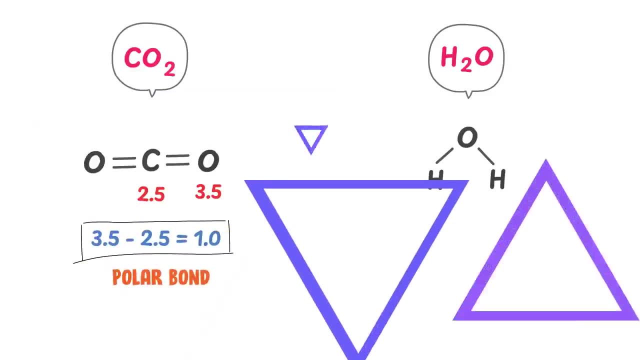 So the bond is polar. As a result of this, partially negative charge appears on oxygen atom and partially positive charge appears on carbon atom. What about the dipole moment of this molecule? Well, the dipole moment is basically like an arrow that starts from the atom partially positively charged and points towards partially negatively. 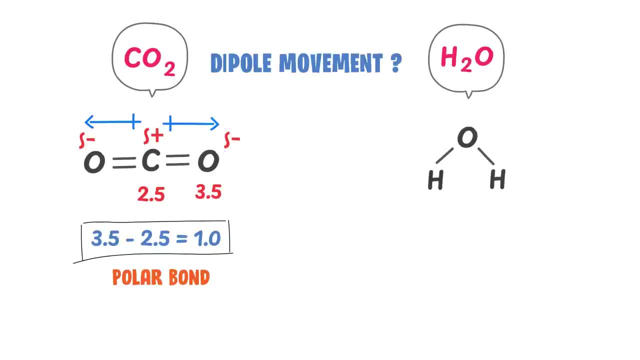 charged atom. Remember that dipole moment is a vector quantity According to the electronegativity difference. oxygen on either side are partially negatively charged and carbon is partially positively charged, So the dipole moment points toward oxygen on either side. The net dipole moment of carbon dioxide molecule is zero, Because the shear period of electrons are equally. 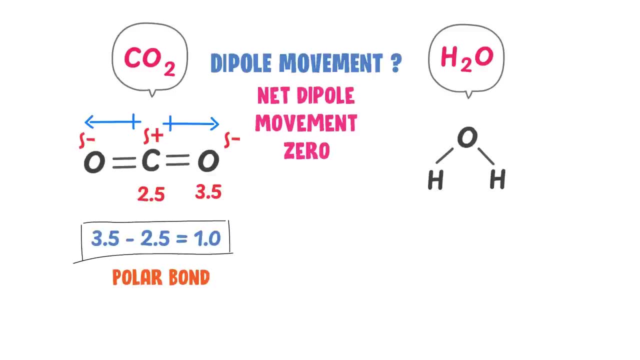 polled by the oxygen atoms on either side. Therefore, carbon dioxide is, overall, a nonpolar molecule. So remember that the bond between carbon and hydrogen is polar, but the net dipole moment is zero. Let me repeat it: The bond between carbon and hydrogen is polar. 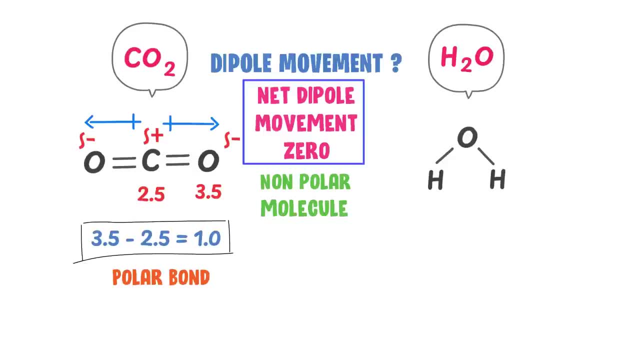 But the net dipole moment is zero. Hence carbon dioxide is a nonpolar molecule In the case of water. firstly, we will find the polarity of oxygen and hydrogen bond. The electronegativity of hydrogen is 2.1 and the electronegativity of oxygen is 3.0. 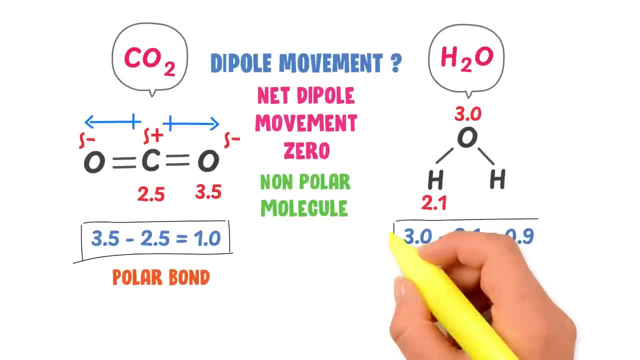 When we calculate its electronegativity difference, we get 0.9.. 0.9 is greater than 0.5.. So the bond between oxygen and hydrogen is polar. Due to this, partially negative charge appears on oxygen and partially positive charge appears on hydrogen. 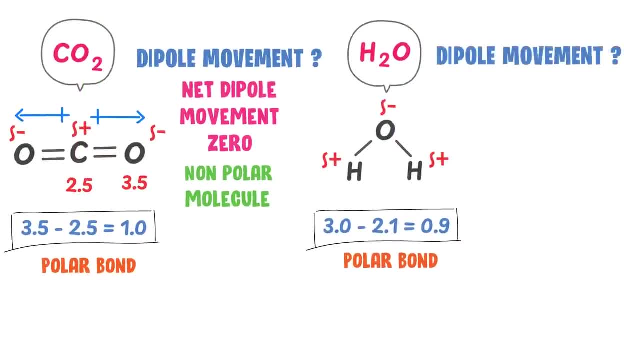 What about the dipole moment of this molecule? Well, the dipole moment, being an arrow, starts from hydrogen and points towards oxygen. Here the net dipole moment is in the vertical direction or in y direction. So the net dipole moment of water is not zero. So we say that.